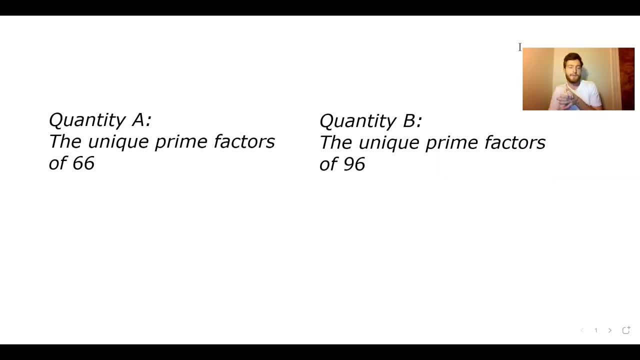 In today's video I'm going to describe how to find the prime factors of any given number and also the divisors of any given number. Many times in the GRE they're going to ask you for the unique prime factors, or distinct prime factors. That means let's say, for example: 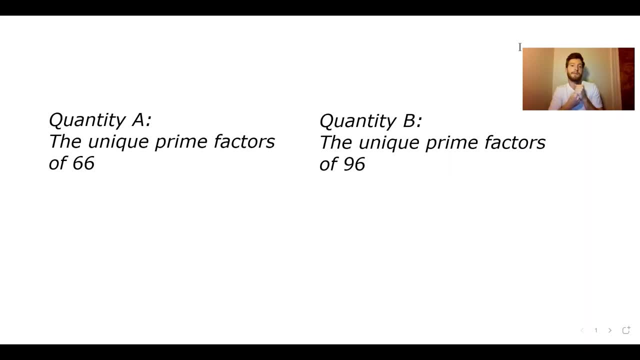 9.. 9 has two prime factors: 3 and 3.. However, it has one unique prime factor that is just 3 itself. That is the only number within the prime factorization. yet the prime factorization is 3 times 3.. So when they say, for example, 6,, for example, it has two prime factors, 2 and 3,. 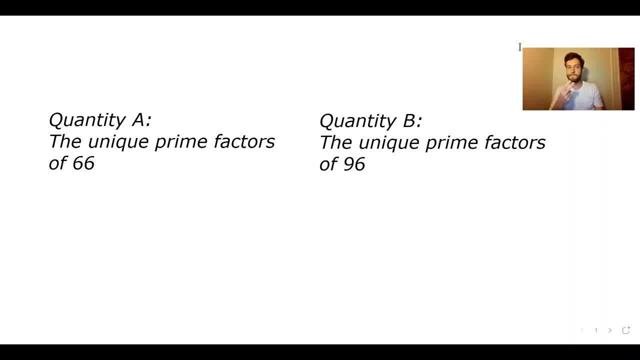 and two unique numbers in the prime factorization: 2 and 3.. Let's look at this quant comparison question: the unique prime factors of 66.. In order to do our prime factorization, we usually divide by a simple number, 2 or 3, hopefully. 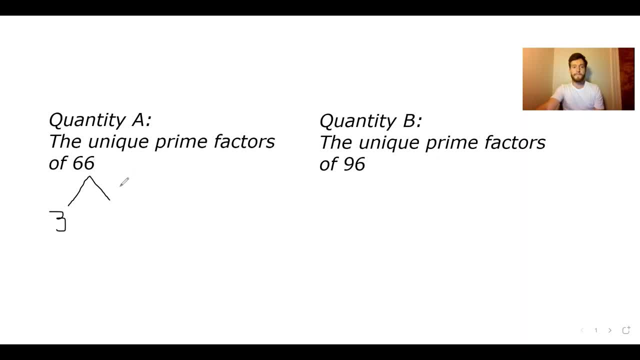 So for this one let's do 3, and that would give us 66 divided by 3 is 22. over here, 22 is going to be divisible by 2.. And then we have 11.. 11 is a prime number, So are these two. So that's our prime factorization. 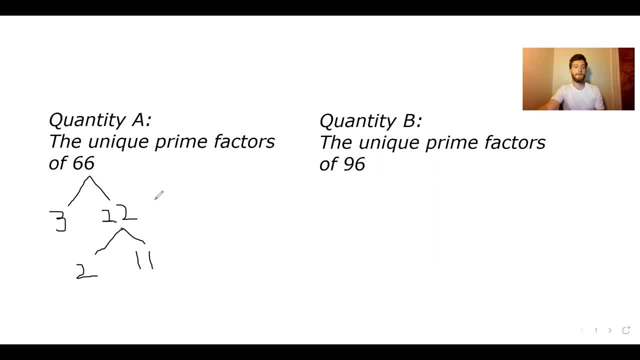 3 times 2 times 11.. Now these are three unique numbers. So we have three unique or distinct prime factors. So our quantity A final answer is going to be 3.. Let's find quantity B. now Quantity B, let's divide it by 3.. 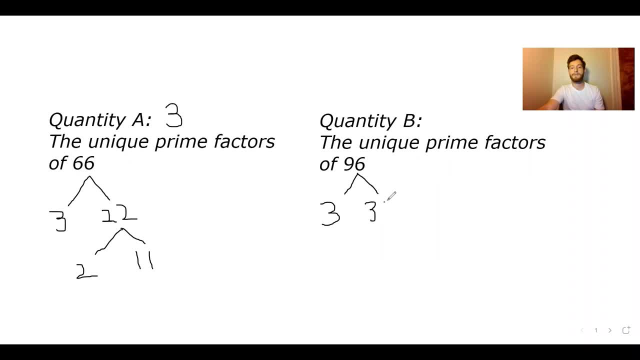 Let's start with b to start. That's going to give us 32 on the right. 32 is divisible by 2, and that's going to give us 16 on the left. 16 is 4 times 4, and 4 is 2 times 2.. So we have a 2 here. 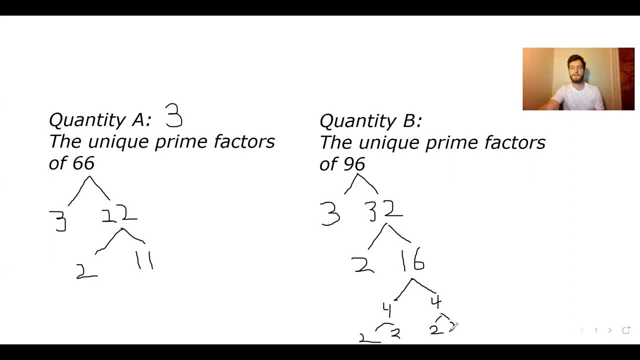 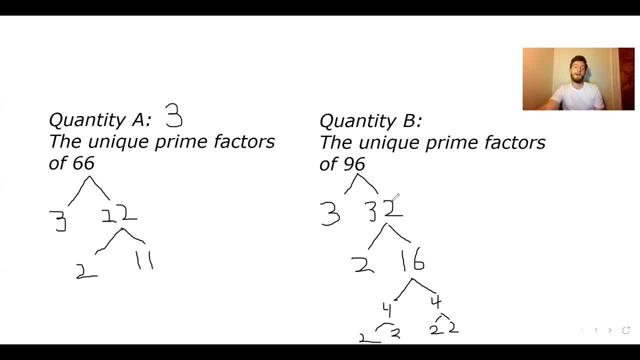 independent problems that you use. there's a very different way of doing a pureveimy here. That's going to give 2 to the fifth power. That is six different numbers right: 3, 2, 2, 2, 2, 2.. But that is. 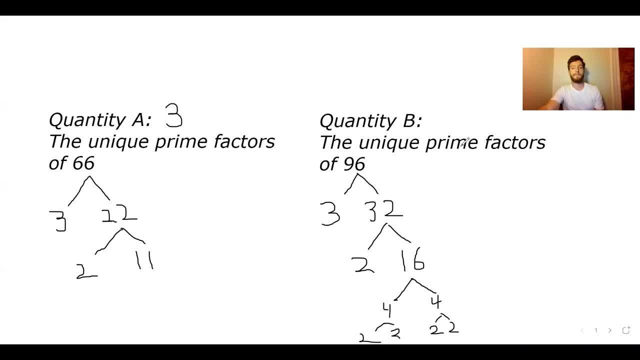 only two distinct numbers or unique prime factors: 3 and 2.. So our final answer on quantity B is 2,, which means quantity A is greater. There are many GRE questions exactly like this, yet they just use different numbers And that's how you would get the answer. 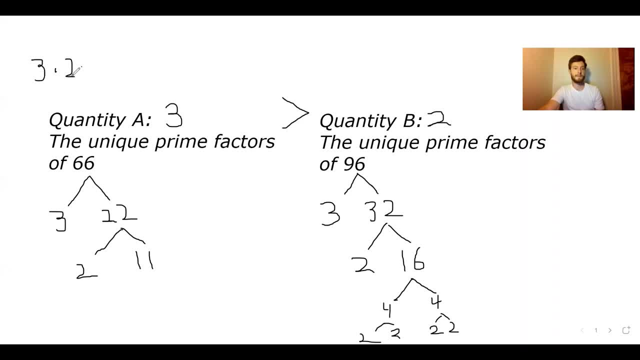 So let's rewrite this very quickly: 3 times 2 times 11, and then 3 times 2 to the fifth power. Yeah, 3 times 2 to the fifth power. 2 and 11, 3 times 2 to the 5th power. It's good to know that for the next one. So the next one. 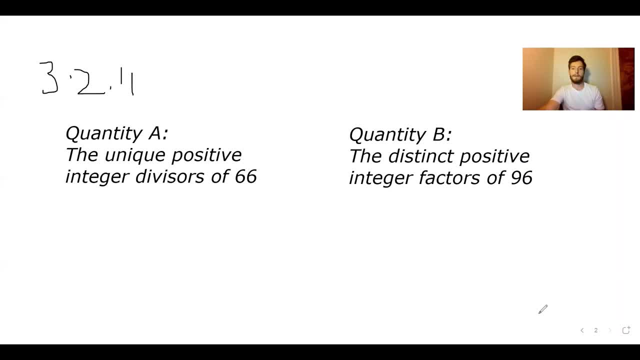 I'm going to just write it out now and then. oops, I already forgot 3 times 2 to the 5th. So this next one is: how many unique positive integer divisors are there of these two numbers? A divisor of 66 is 3,, 2, and 11,, but also a divisor of 66 would be. 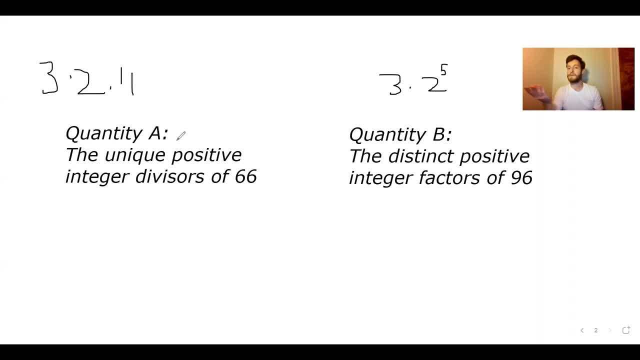 33.. 66 divided by 33 is 2, or 22.. So divisors do not have to be prime, Factors don't have to be prime. That's why there's the prime and then there's the divisor. So divisors do not have to be prime, Factors don't have to be prime. 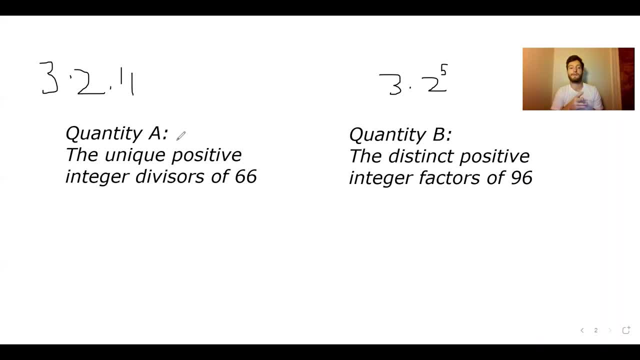 In front of the word prime factor itself is the same as a divisor. On both of these I chose different wording, just so you get used to them. They're asking the same exact thing. Sometimes they say unique, sometimes they say distinct, sometimes they say divisor. 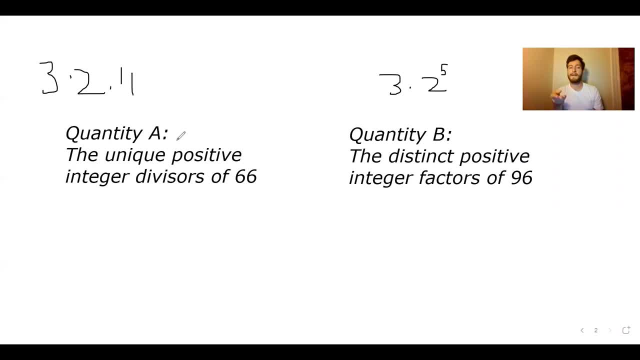 sometimes they say factor- In order to find the unique positive integer divisors of any given number, we first do the prime factorization, just like we did before. But with the prime factorization there is an equation we can use to find the distinct positive integer factors, and it goes like this: